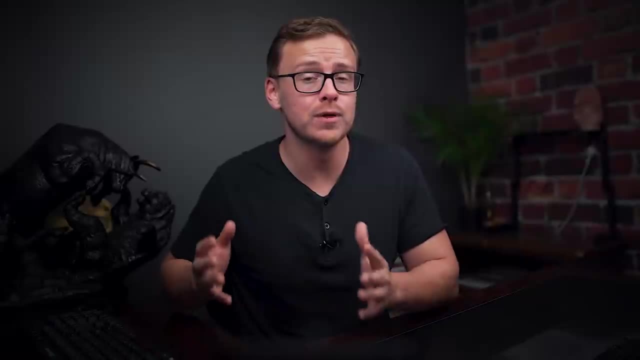 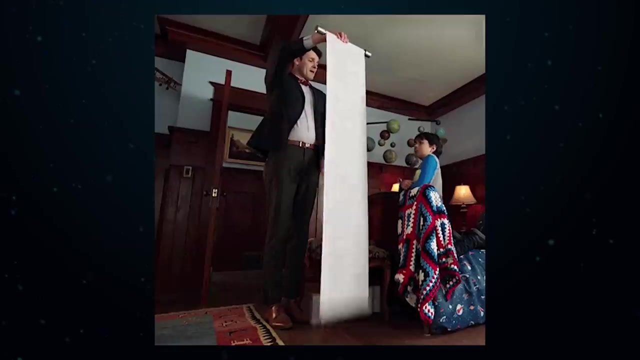 What's happening. It's Shane here, and in today's video we're going to be talking about the top five personal finance tips for college students. Now this is going to be a list of the top five things that I wish I would have told myself back when I started college, and the top five things. 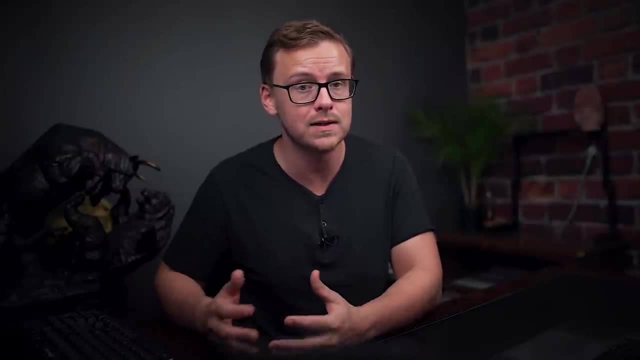 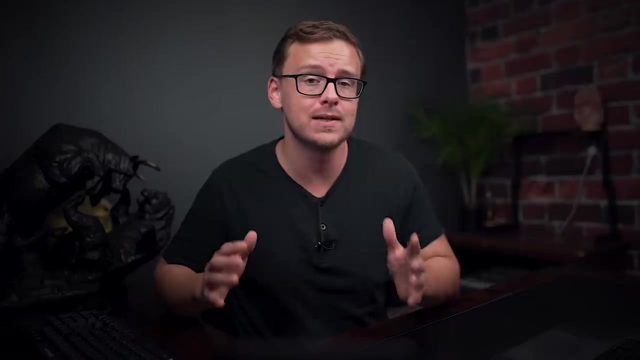 that I think are the most important when it comes to personal finance for a college student, And if you are able to get these five things down, it is going to make a world of difference. It's going to be like night and day and you're going to make the rest of your life a lot easier. But before we 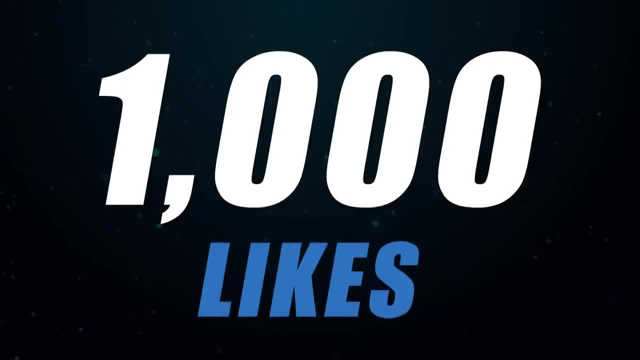 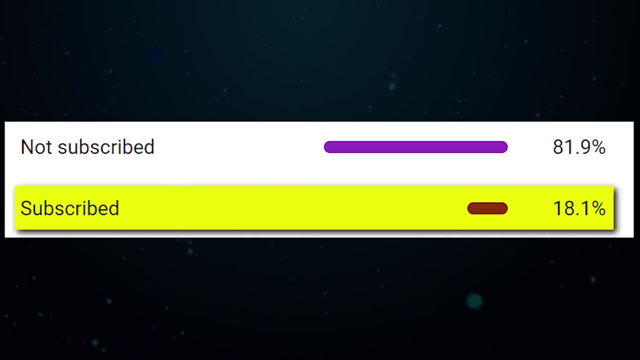 get into that. let's make sure to gently tap that like button. Let's set a goal for a thousand likes on this video. Hit the subscribe button. Only about 20% of you are subscribed. We could do better than that. Come on now And also ring that notification bell so that you never miss out on a video. But 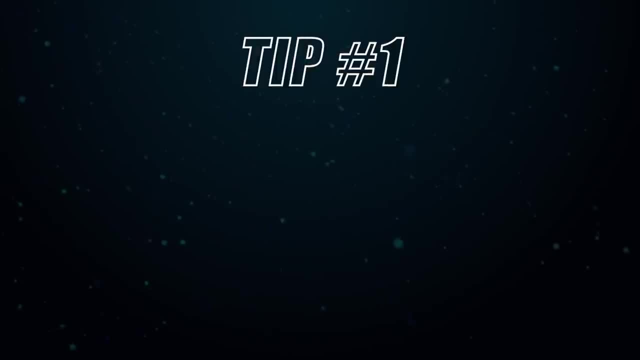 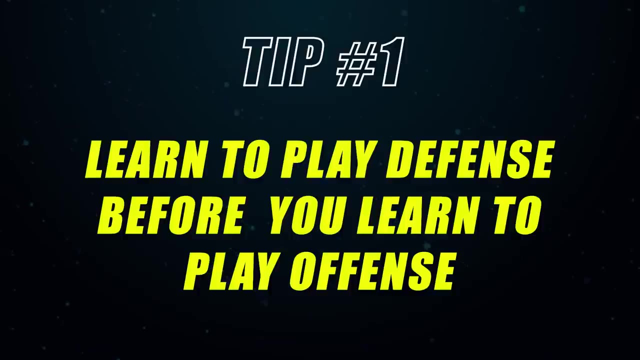 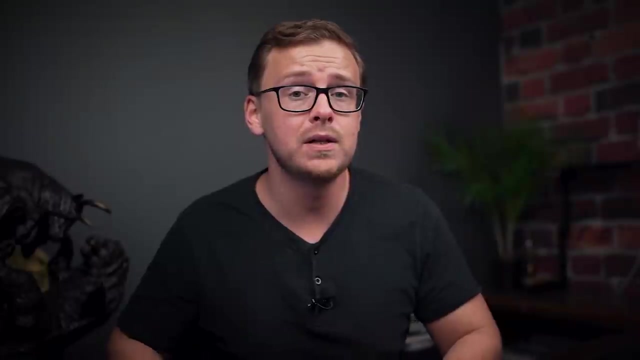 anyways, let's get into it. Number one on this list is to learn to play defense before you learn how to play offense Right. and I'm not talking about basketball or football, This is just a money metaphor. So basically what this means is learn how to save and budget your money Right. so if offense is 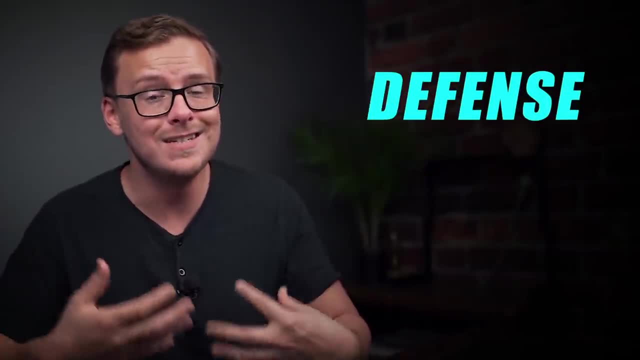 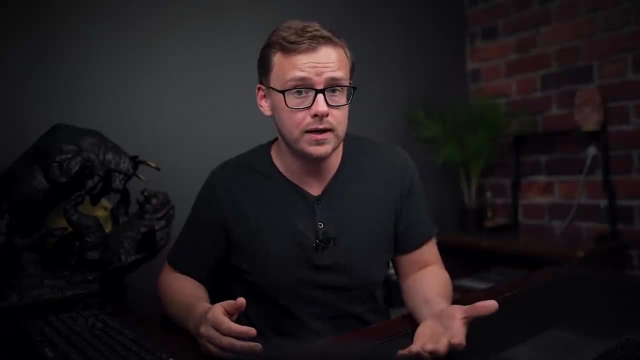 making your money and then also investing your money, then defense is saving money and learning how to budget, And the only problem with offense is during a lot of your life- while you're young specifically, you don't really have all that many opportunities to make money. Usually you have to. 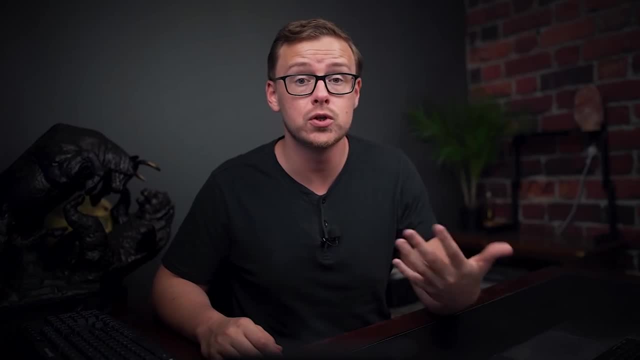 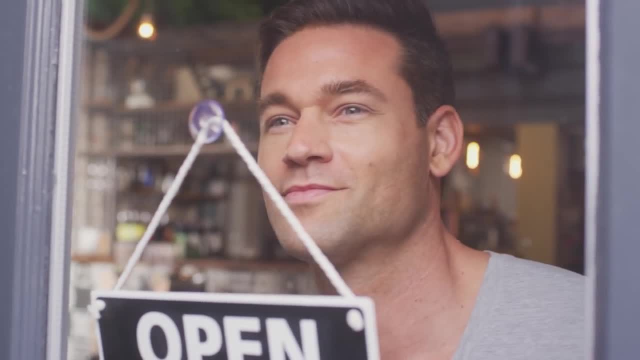 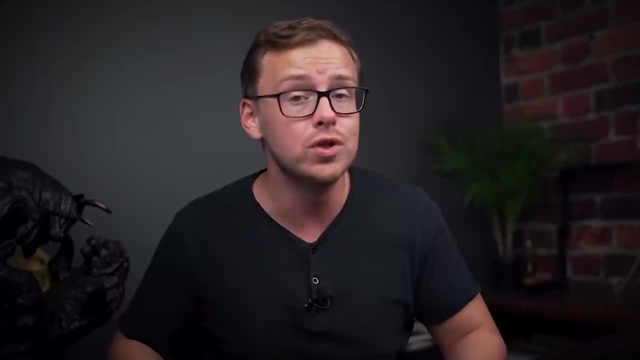 have to start a business, and usually the first few years you're not going to be making very much, So it's very difficult to learn how to make money, and even more difficult to learn how to invest it while you're young, just because you don't have all that many opportunities. But what is just as 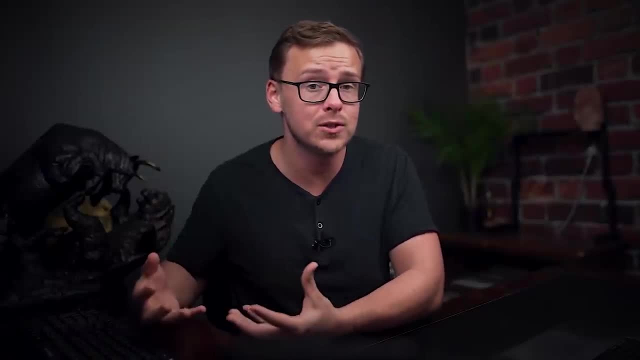 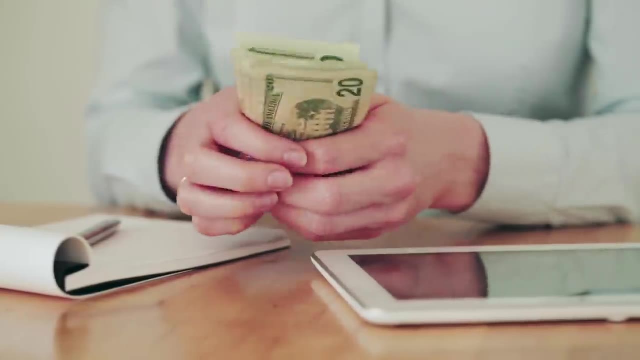 important as learning how to make money and learning how to invest your money is learning how to keep it Right, learning how to budget so that you can actually save money and keep the money that you make and invest it. So that's number one. Number two is to learn how to make money and 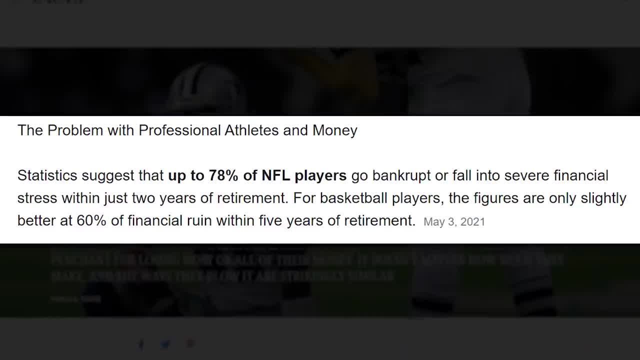 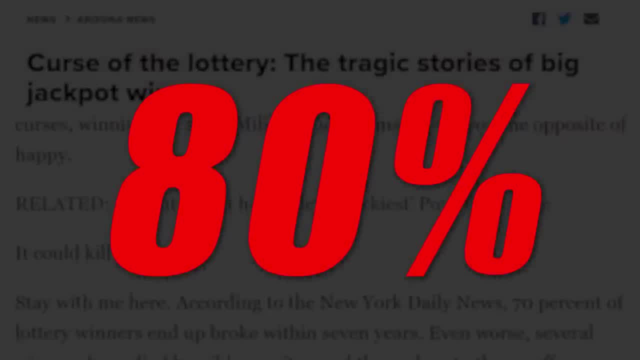 invest. And just to prove this, in case you don't believe me, 70 percent of professional athletes end up going broke and 80 percent of lottery winners end up filing bankruptcy. These are people who have millions and millions of dollars. They have so much money that they could probably have like. 10 or 20 or 100 different people retire on the amount of money that they make during their career or, in the case of lottery, how much money they get from the payout. And yet, in many cases, they still end up losing it all and they go bankrupt. Why? Because they don't have the money They don't have. 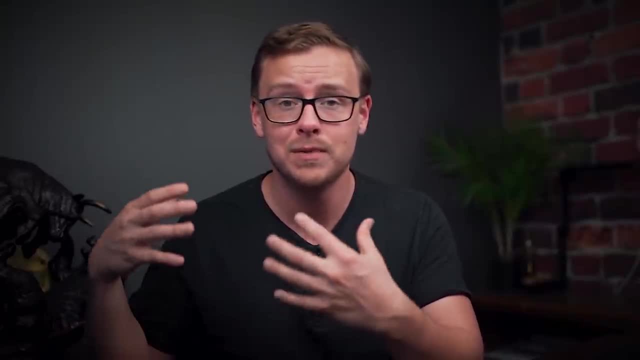 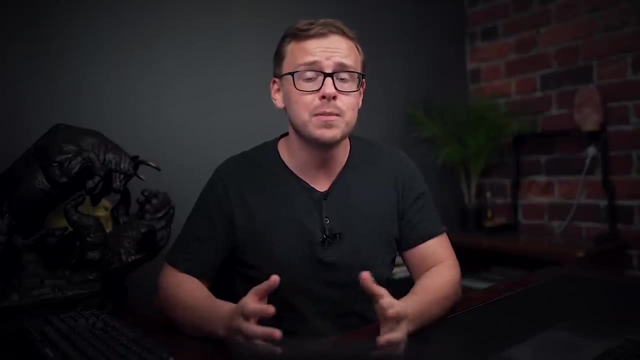 the money. Why is this? Because they had the offense part down. You know they made all that money but they didn't have the defense part down. They didn't understand how to budget and save. So the defense part is something you can practice at any time during your life. You can learn the basics of 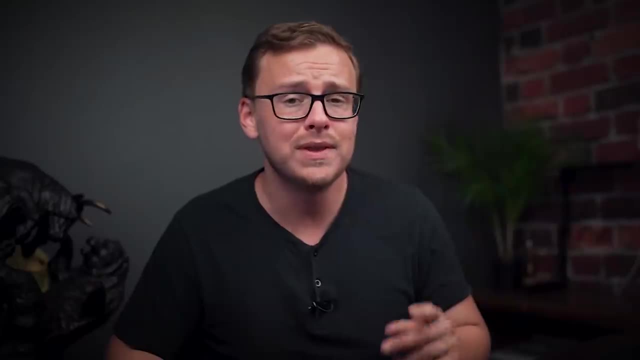 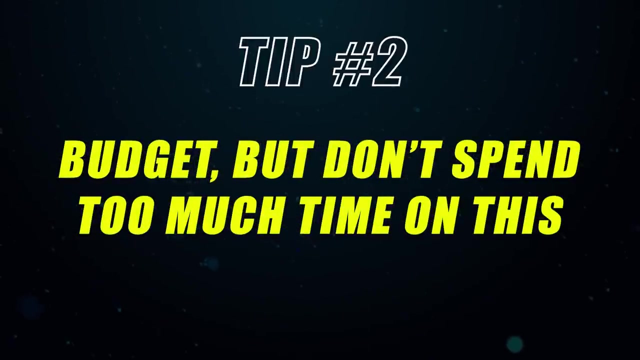 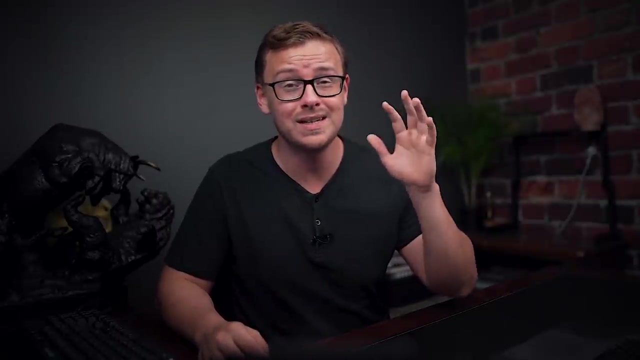 budgeting and you can learn the basics of saving money. But that brings me to number two on the list, which is budget, but don't spend too much time on it. So I see a lot of YouTube videos where people basically get super, super detailed with their 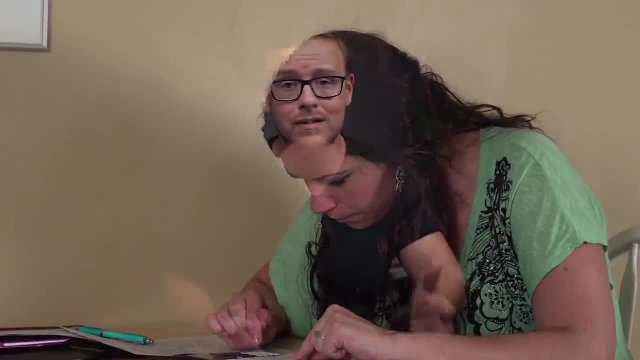 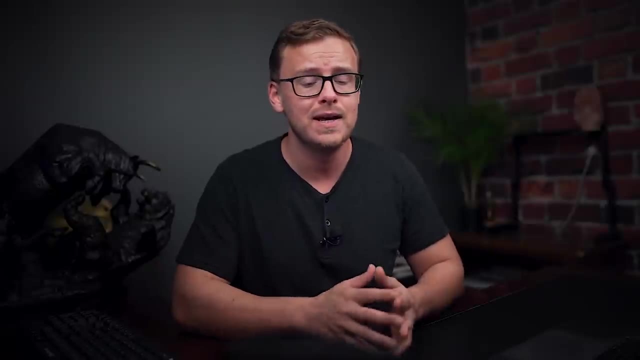 budget, Like they're tracking every single penny that goes in and out of their account and out of their pocket or their wallet. And some people will even say: I spend like an hour a day doing my budget, And to me that is just absolutely ridiculous. Avoid time wasting tasks where you're trying to 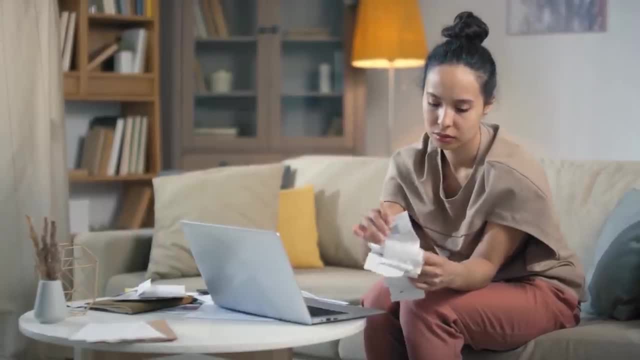 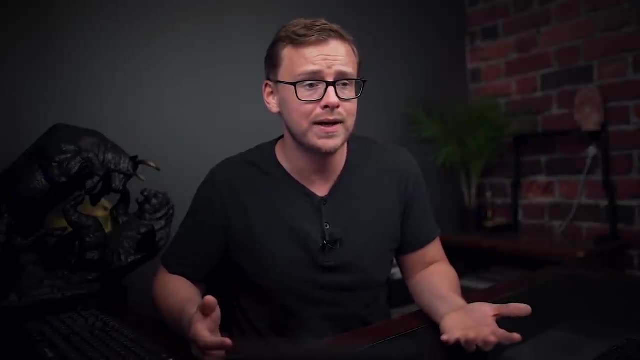 manage your money too much. So this would include budgeting, of course, because you know if you spend like an extra day on your budget in order to save like an extra dollar to per day, I mean that's really not going to make that much of a difference. you could just use that amount of. 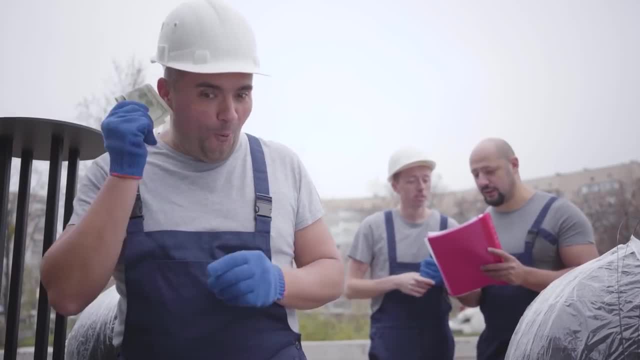 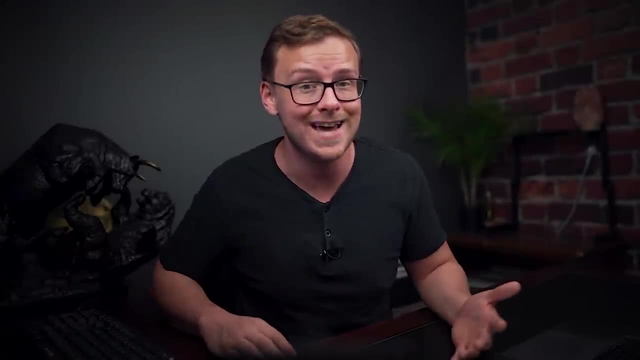 time that you were budgeting And like pick up extra hours or you know, go do some kind of side hustle And even if you're making like 510 bucks an hour, you're gonna end up making more money doing things that way. But this also includes things like extreme couponing, which, in my opinion, is usually 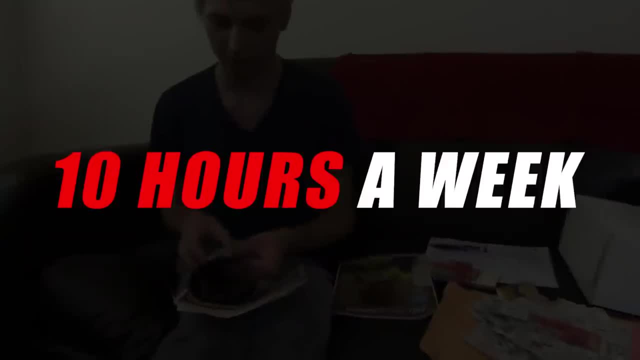 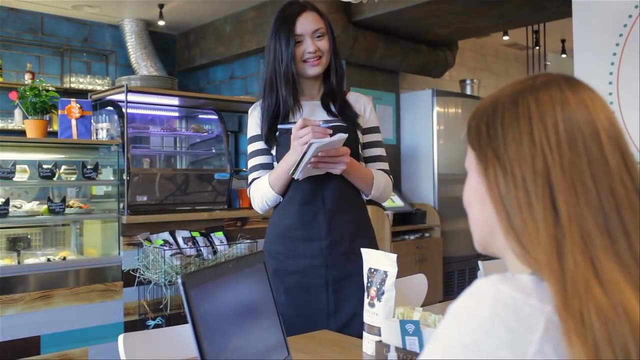 going to be a total waste of time. You know you spend like hours a week in order to end up saving $50, that's $5 an hour. You could have just worked like a minimum wage job and you would have made a lot more than that. Now, that's a great thing to do. 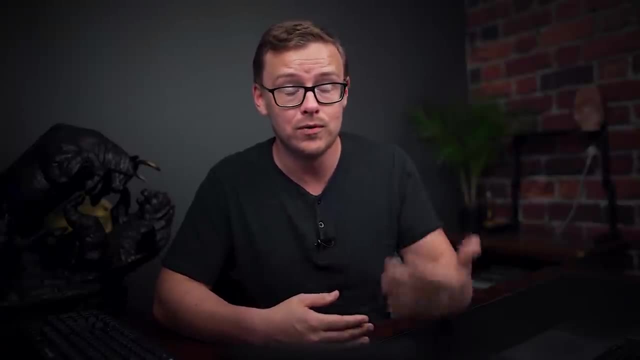 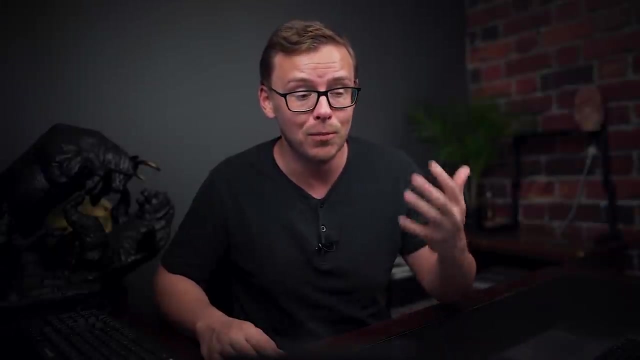 if, for whatever reason, you don't have access to a job. but if you're able to work a job, you can just work extra hours, do some kind of side hustle, do Uber, you know anything like that, and it would be more worth your time than spending all this time sorting through different magazines and 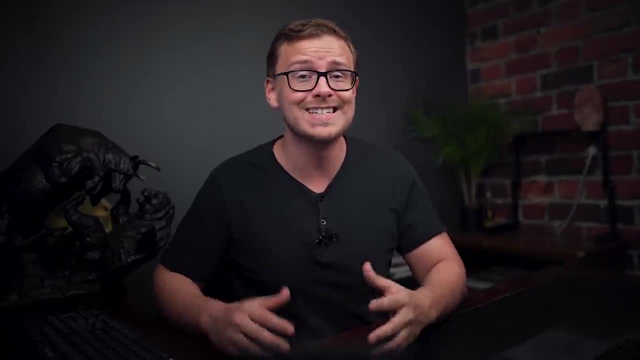 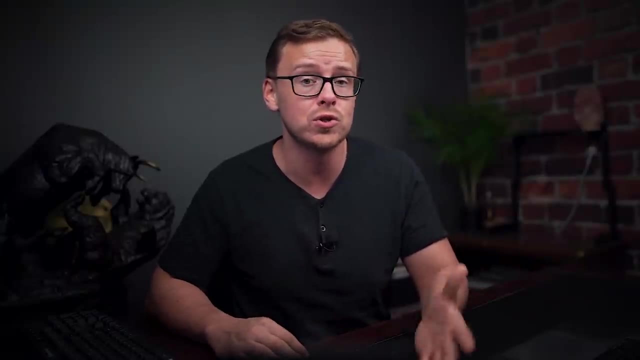 newspapers and stuff like that. Another example of one of these things is wasting too much time thinking about credit card points. So there's like a very basic credit card strategy that you should understand. You know I have a few credit cards and I use them strategically to, you know, save. 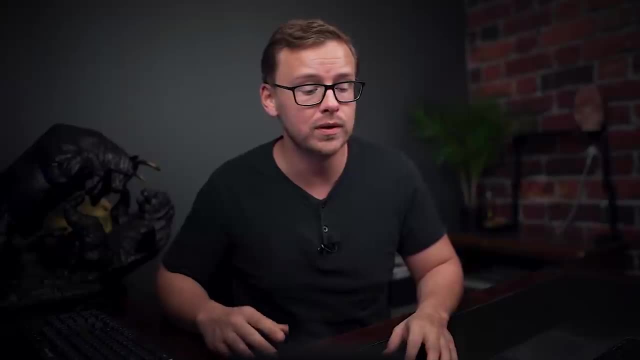 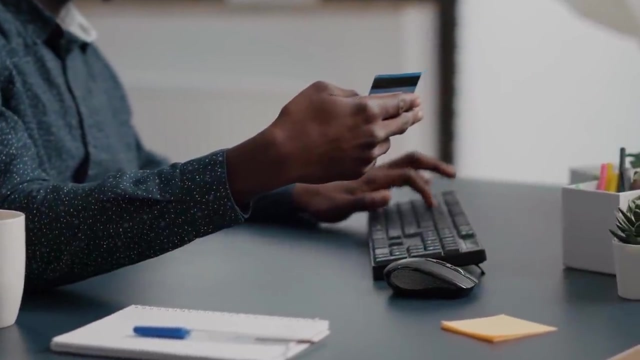 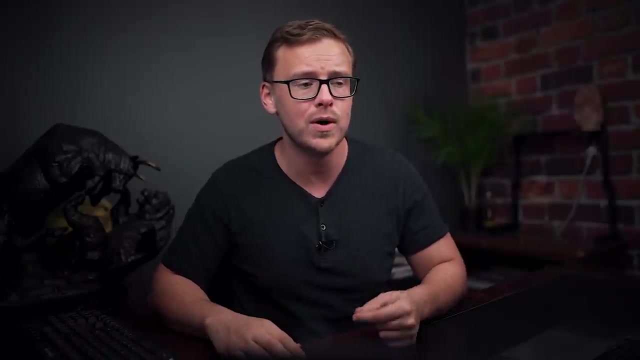 money. but some people just go way overboard with it and they have like 20 different credit cards and they're monitoring like, oh, during January, February and March, this one is gonna, you know, give me 3% Back on gas, which is a little bit better than the 2.5%. So they're like constantly like switching. 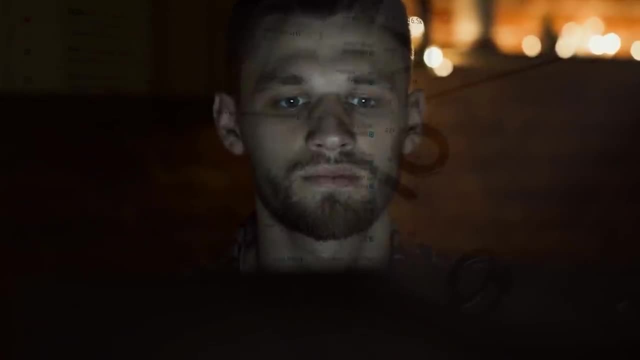 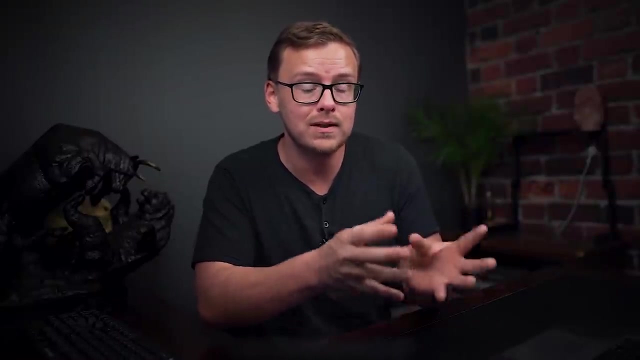 their credit cards out and just they spend all this time on like credit card forums reading about other people's experiences, and they could have just taken all that time that they did that and learned a skill that they could have used to made like way, much, way more money, right. 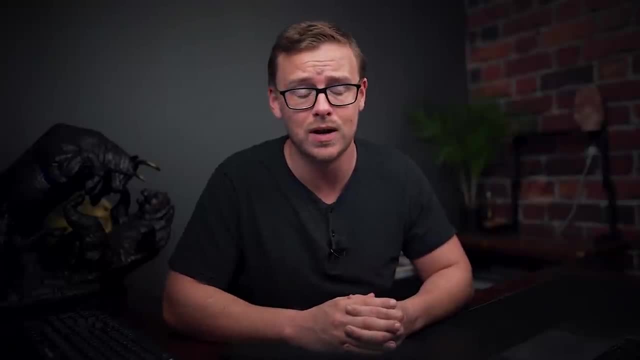 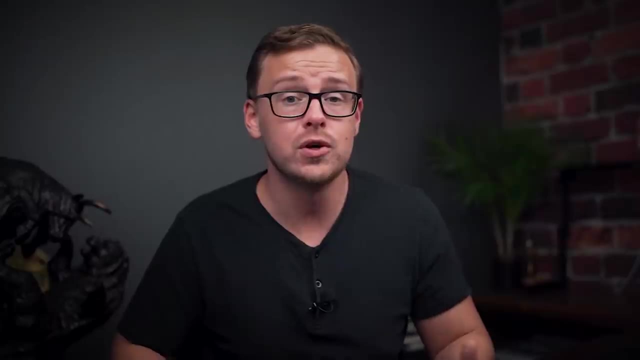 And instead they ended up saving like maybe an extra hundred bucks a year or something right, But they could have, like, like I said, learned a skill to to make more money, Or they could have just worked extra hours. So I'm all for credit card points and everything like. 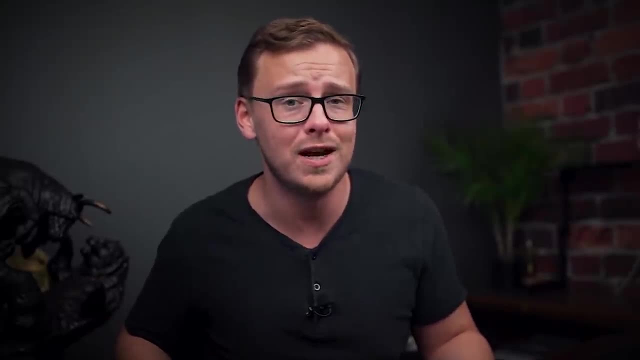 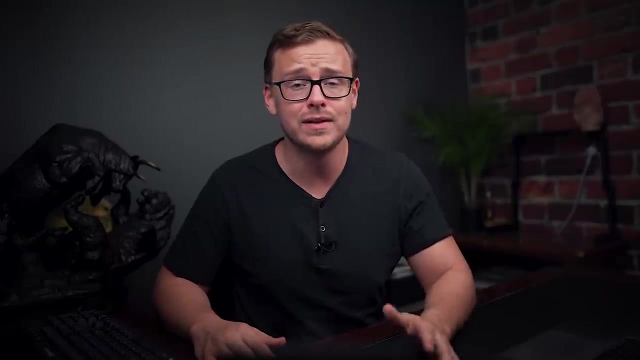 that You should definitely do that, but do it smart, Don't waste too much time on it. Just get the basics down. you know, just get a couple of really good credit cards and you are good to go. And there's honestly a lot of other things that I could use as examples of things where you're 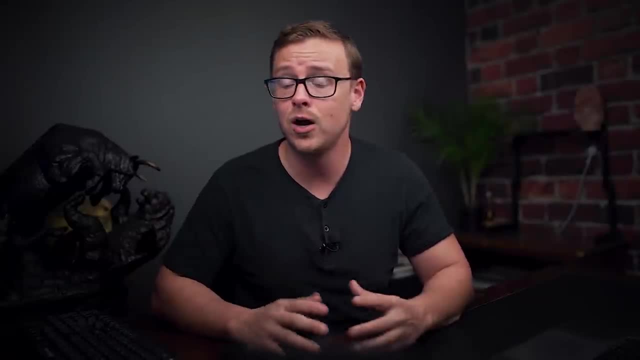 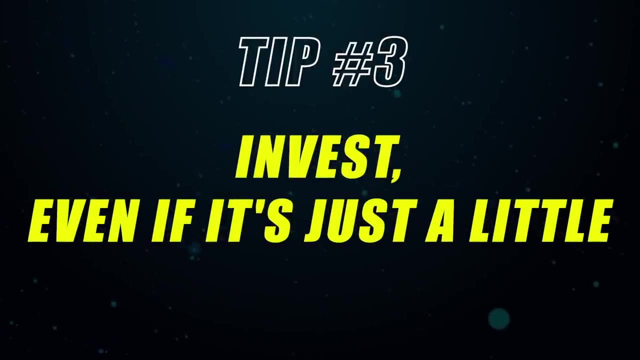 you know wasting your time doing too much of something, but yeah, I'll go ahead and leave it at that. Number three on the list is going to be start investing as early as you possibly can, Even if it's just a tiny amount of money. 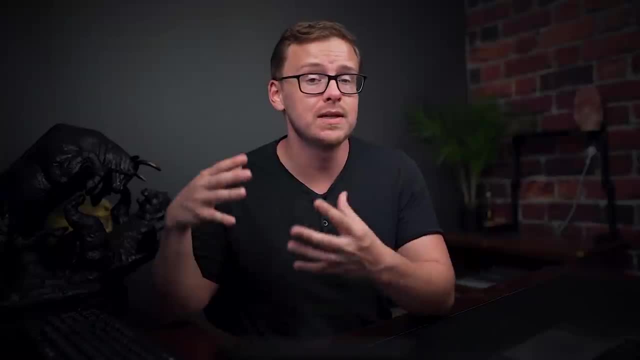 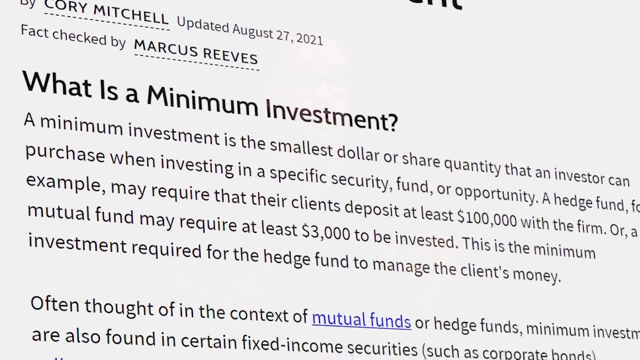 It used to be that most people did not start investing until they were in their thirties, And a significant reason why that was is many of the brokerages had minimum amounts that they required for you to open an account, So it would be something like $5,000,, $10,000, et cetera. 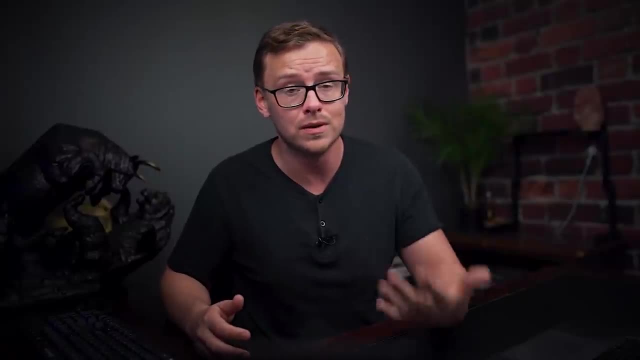 And the truth is, a lot of people, especially these days, with student loans and house payments, et cetera, they aren't going to start investing until they're in their thirties, And a significant reason why that was is many of the brokerages had minimum amounts that they required for you to open an account. 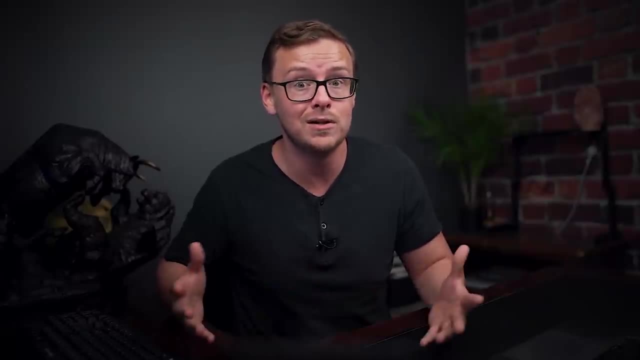 So it would be something like $5,000,, $10,000, et cetera, And a significant reason why that was is many of the brokerages had minimum amounts that they required for you to open an account going to have $10,000 of disposable income for a long period, a lot of the time, until they're in their thirties. 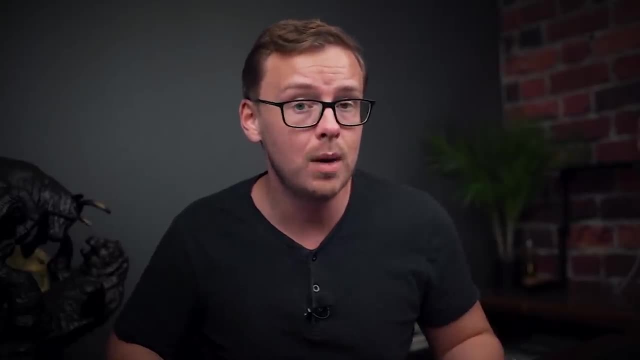 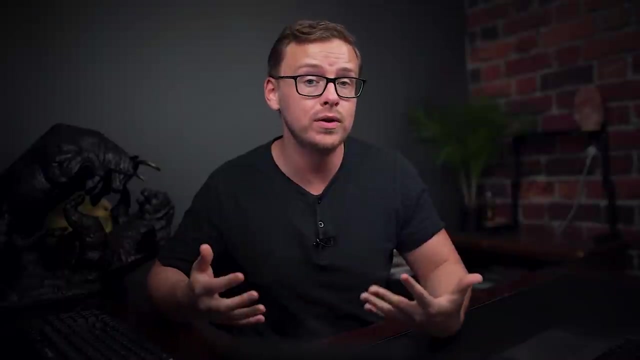 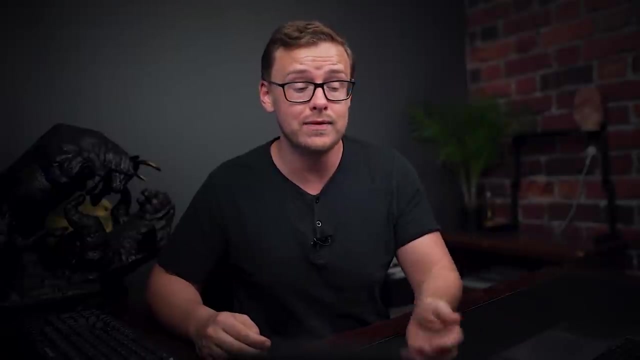 But these days there are so many different investment options for you. You could literally pick up your phone and download an investment option right now and start investing, And not only would you have the incredible power of compound interest on your side, which is basically where you know during your lifetime. 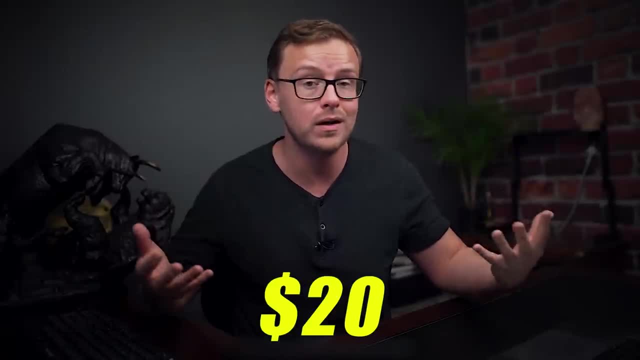 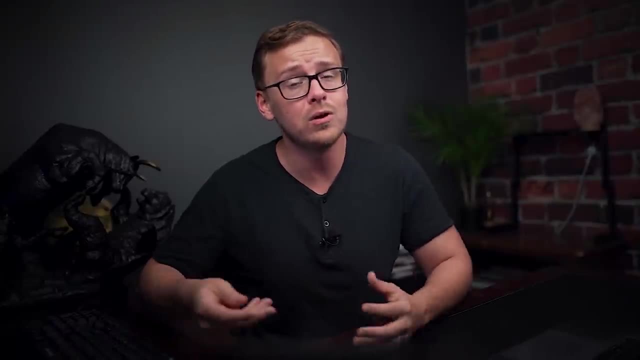 $1 is going to turn into like $10 or $20 down the line if you invest, If you invest it long enough, whereas if you wait until your thirties, forties or fifties to start investing, that $1 might only turn into like $5.. 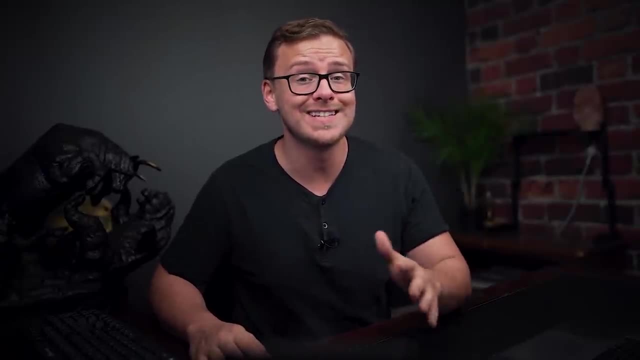 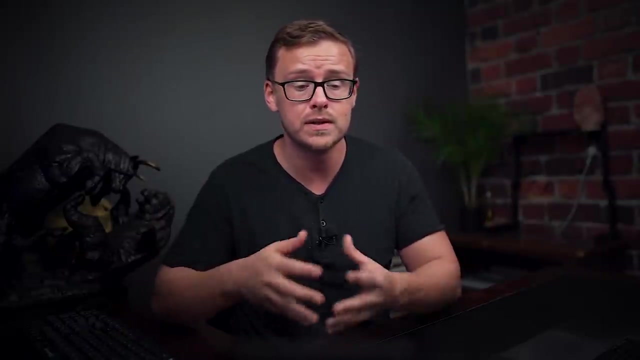 Now, the magic of compounding investing is super important and I think that's awesome, but I think most people have heard about that before. You know, if you invest like $500 a month into a Roth IRA, for instance, all the way through your lifetime you are going to be retiring as a tax-free millionaire. 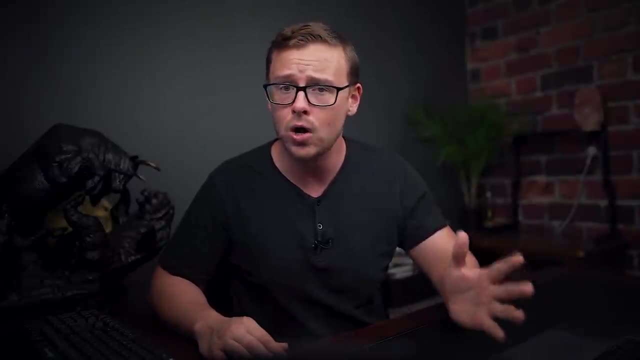 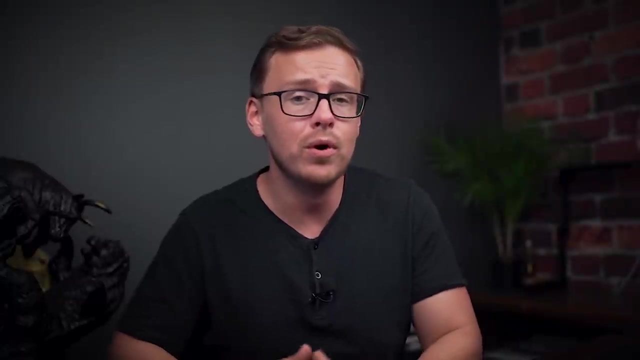 This has been proven over and over again. There's Roth IRA calculators all over the internet. You can do the calculation yourself. You are going to retire with millions and millions of dollars, But I think, even more than the power of compound interest, it's just the simple fact that you get started investing right. 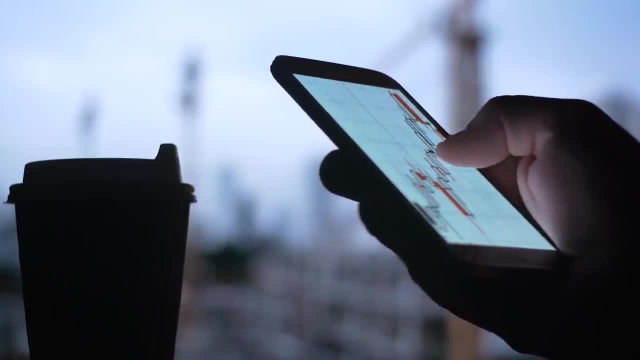 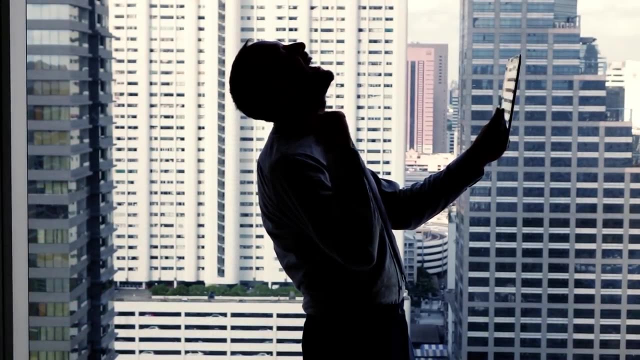 When you open up your phone and you see that your investments are going up, like, oh, you open it up, You see your investment going up, You get this a little adrenaline rush. It feels really good And there's really just a psychological aspect to getting started investing as soon as you can. 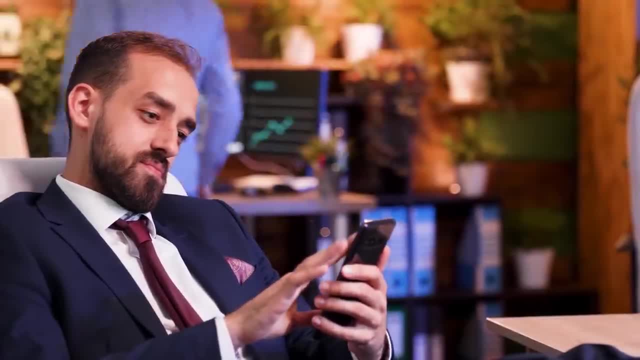 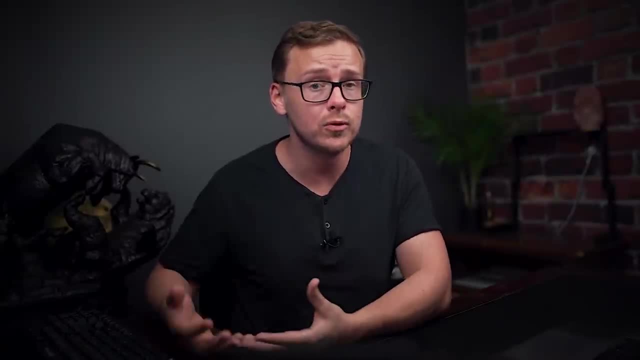 And it gets kind of addicting, And that is a very good addiction for you to have, as long as you invest wisely, of course. So the sooner you start doing it, the sooner you're going to get more comfortable with it, And that is going to lead to you really getting into investing. 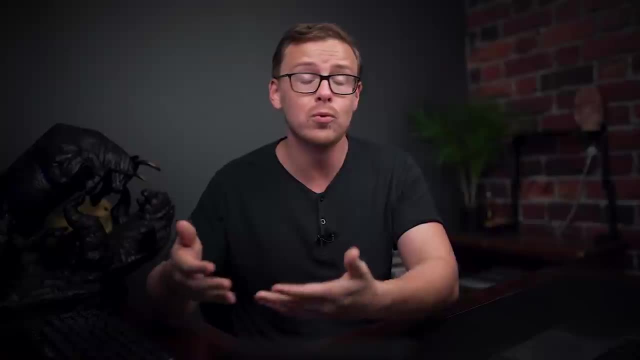 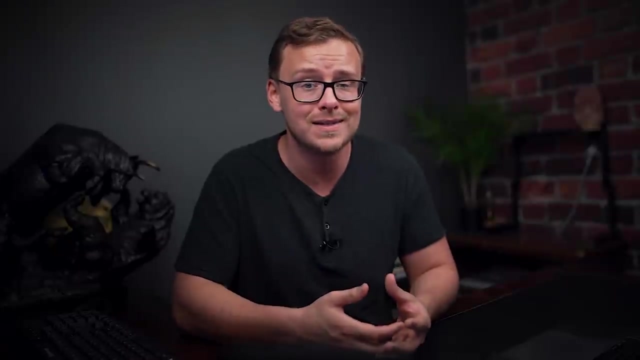 And then it's going to be so much easier for you to do things like number one and number two, which is save and budget, Because the more you save and the more you budget, the more you're going to get to invest, And it's also going to be easier for you to do the next two on the list. 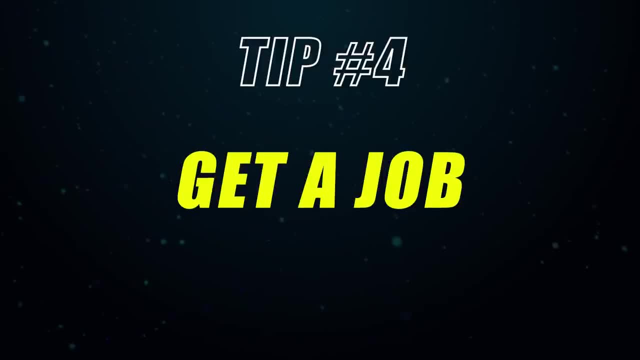 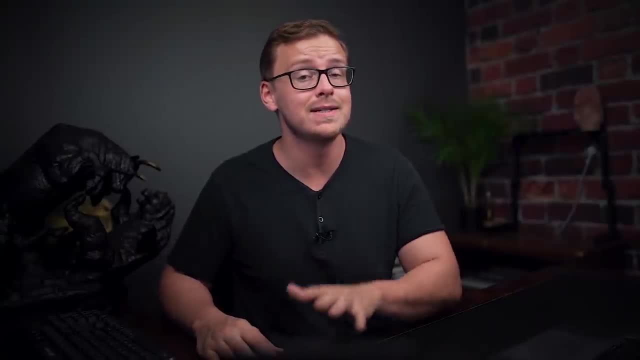 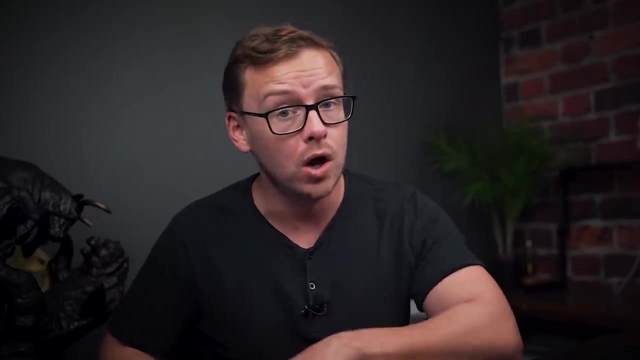 And the next one is going to be number four. Number four: get a job. Right, I know I probably sound like a boomer saying this, but this is a very important thing for you to do during college And, honestly, if you can, during high school, I would say during college, getting a job is even more important than having good grades. 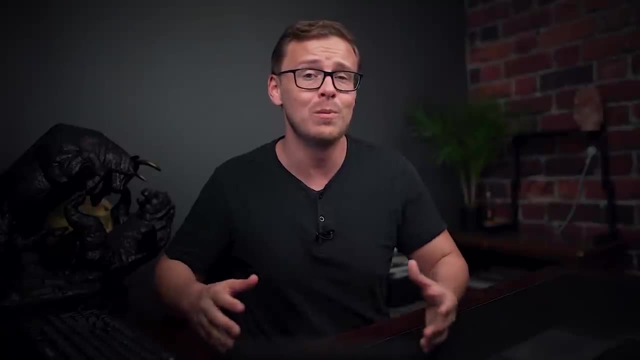 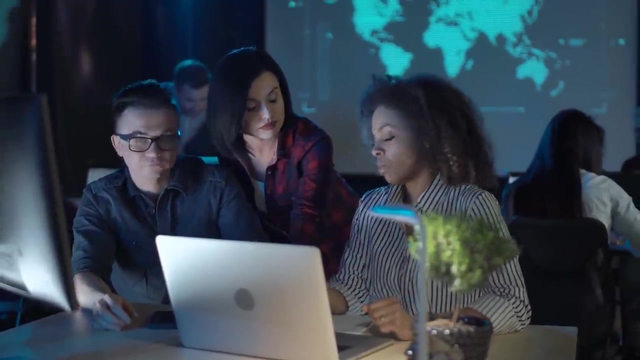 And the reason for that is because if you don't have work experience, it's so much more difficult for somebody to train you, And I know from personal experience. I've trained people who worked while they were going to work. I've trained people who worked while they were going to school. 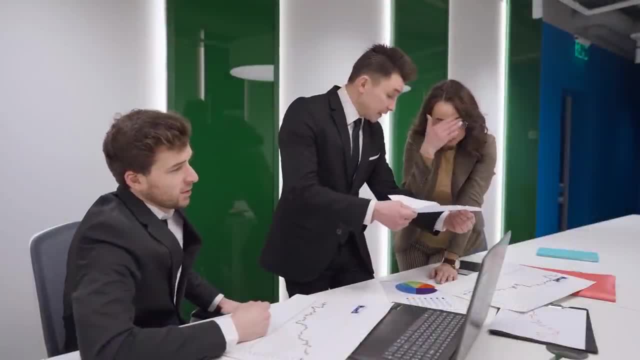 And I've trained people who didn't work while they were going to school. It was their very first job And the difference is night and day And it wasn't because, you know, the people who worked were much smarter than the people who didn't work. 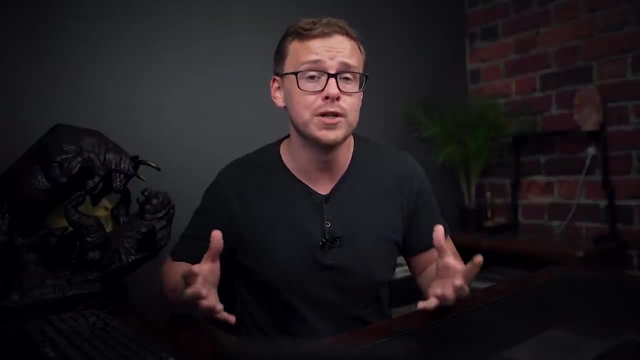 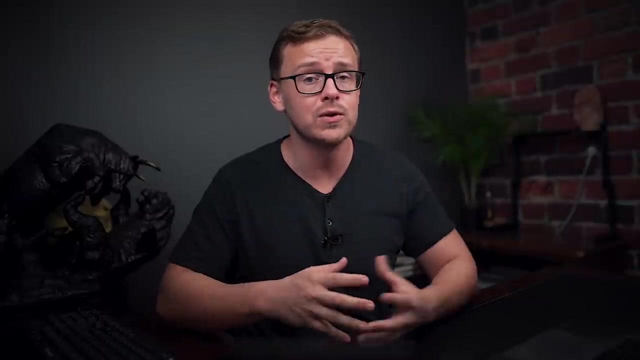 It was simply just experience. It is so much more difficult to train somebody who has zero work experience versus somebody who has some, And hiring managers, business owners, et cetera, they all know this. So not only are you going to learn key skills, 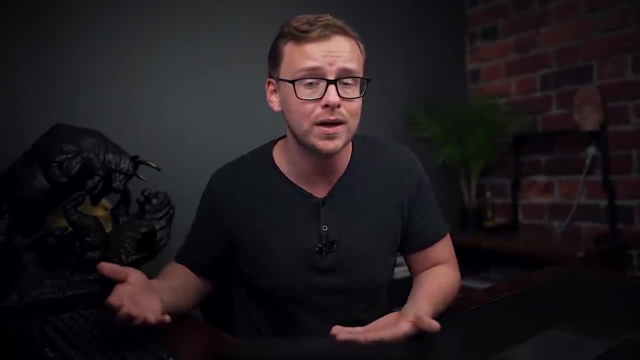 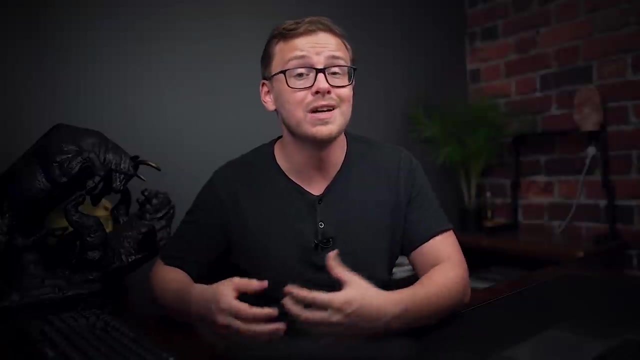 And these are kind of soft skills You can't really learn out of a book. You just have to be there, You have to do it. It's on the job training type of skill sets. So not only are you going to learn those skills, but on top of that it's going to look so much better on your resume when somebody sees that you were working during college. 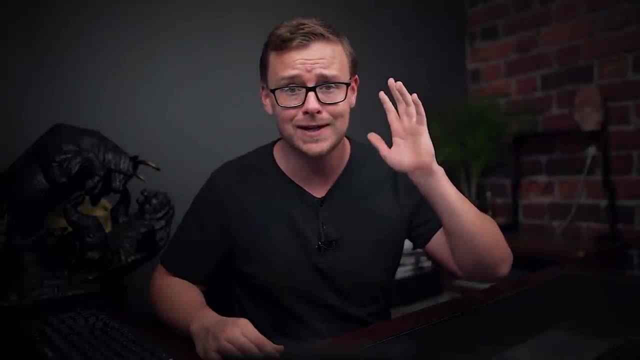 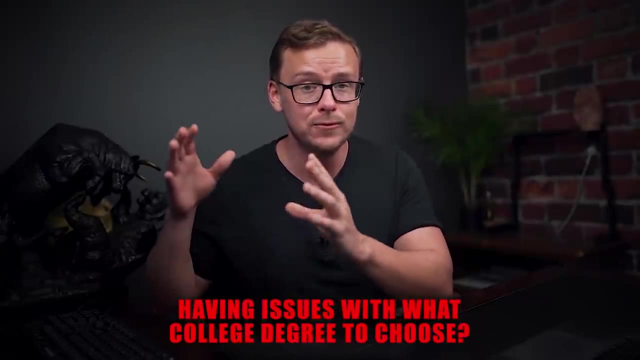 So even if you can pick up like seriously, just like, even if it's like a half shift every two weeks or a half shift every month, as long as you get to say you worked part time during college, it's going to look a heck of a lot better. 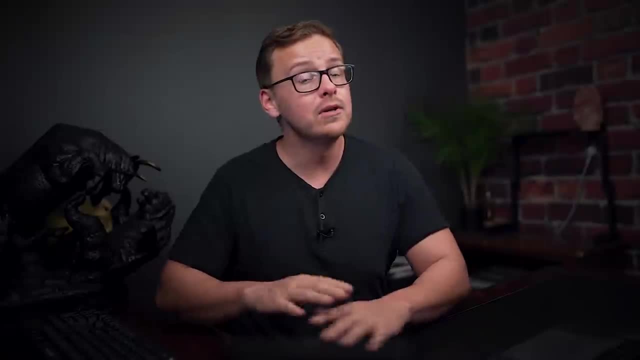 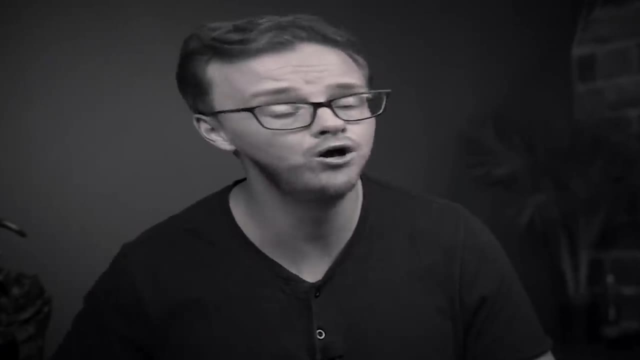 Than someone who didn't work at all, And even if you're somebody who's like you know what? Shane, I'm going to college, but I don't plan on getting a job. I'm going to be an entrepreneur, Okay. 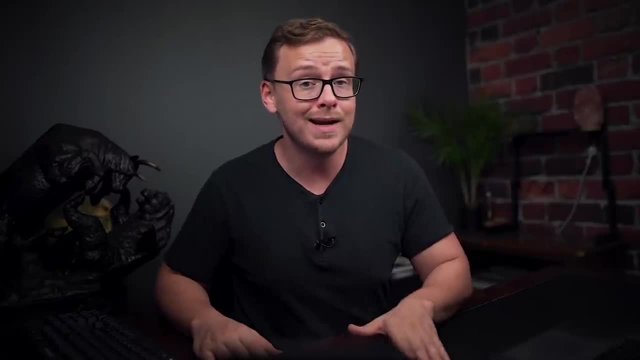 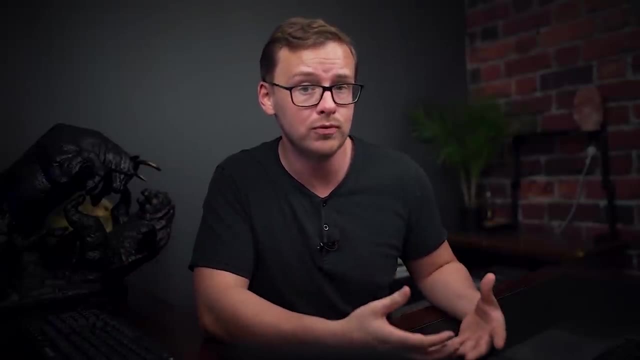 I'm never going to work for anybody else. I think that's a really bad mindset, because how are you going to be able to be a good boss yourself if you've never been an employee before? right, Like it's so much easier for you to put yourself in somebody's shoes if you've been in their situation before. 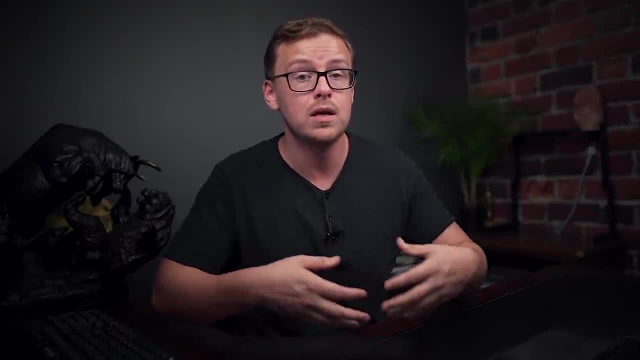 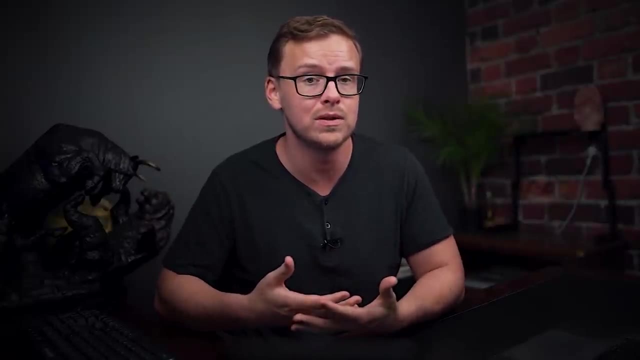 Like it's so much easier to be a good manager if you've had a bad manager, or you maybe you've had a good manager before and you kind of have seen the contrast between those two. So even if you get a job, and it's kind of a crappy job, you don't really enjoy it. 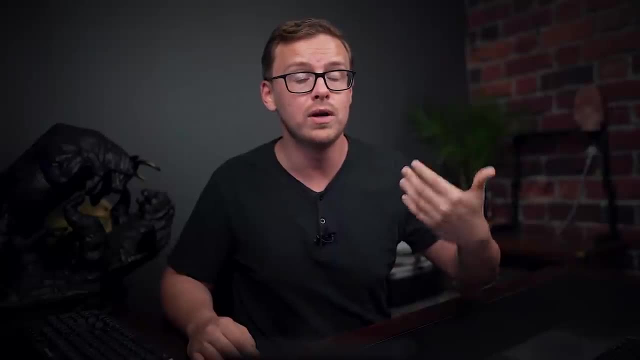 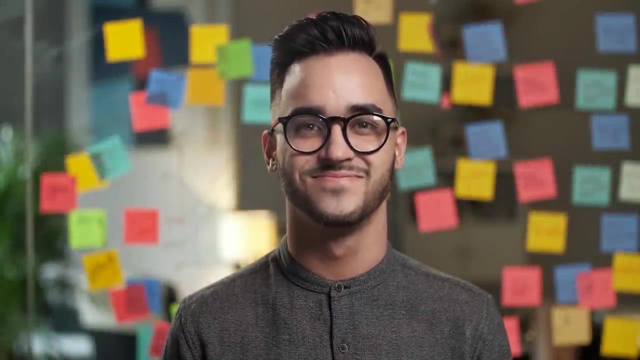 That's going to set a bar for you, And so in the future, if you get a better job, it's going to feel a lot better. You're going to actually appreciate it because you know that it's better. And then on top of that, you're just going to learn so much. 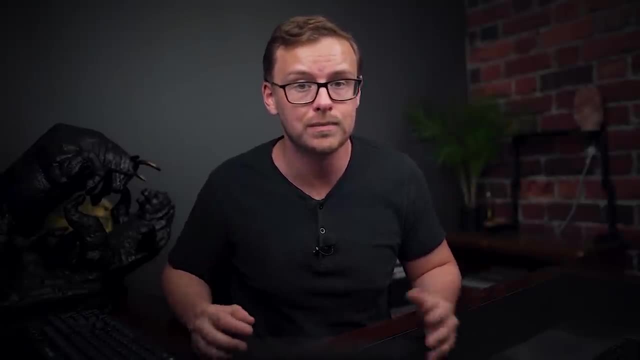 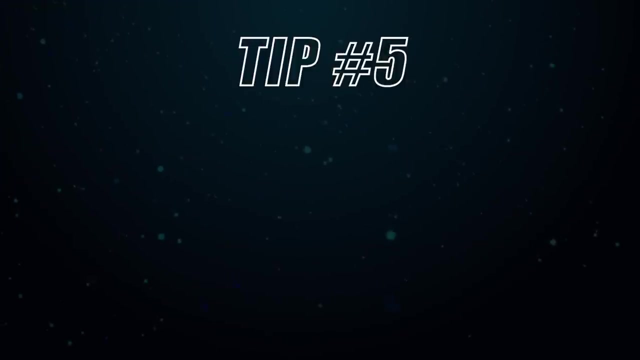 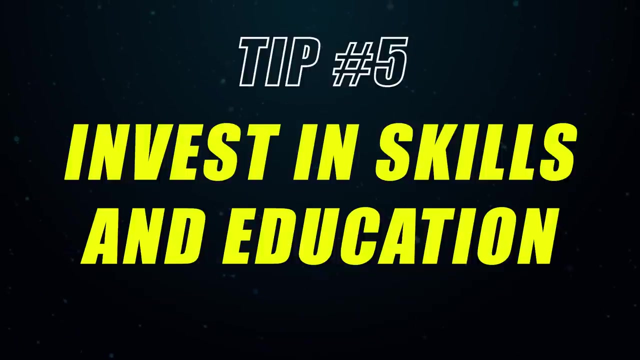 No matter what, No matter what direction you end up going. So definitely get a job during college, without a doubt, No brainer, Just do it. Number five on the list is going to be to invest in skills and education. Now, education is one of those things where college used to have a monopoly on it, right? 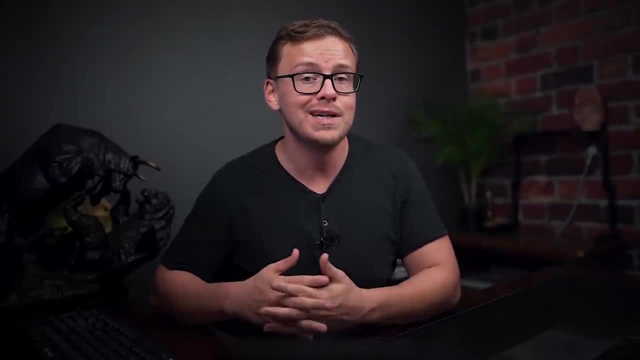 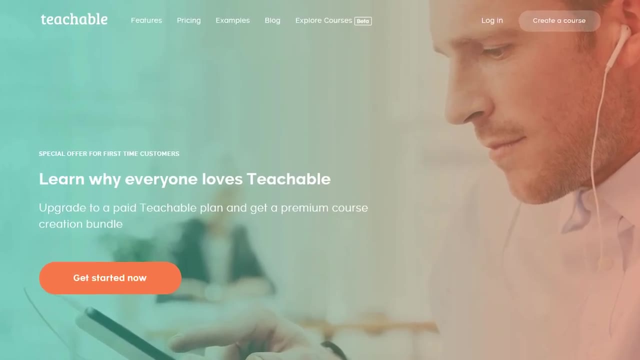 Pretty much the only place you could get educated was college, But it's no longer like that right. There's so many different areas. There's so many different areas that you can get educated in. There's lots of different websites out there where you can take courses from. you know people who are pros at whatever they're teaching. 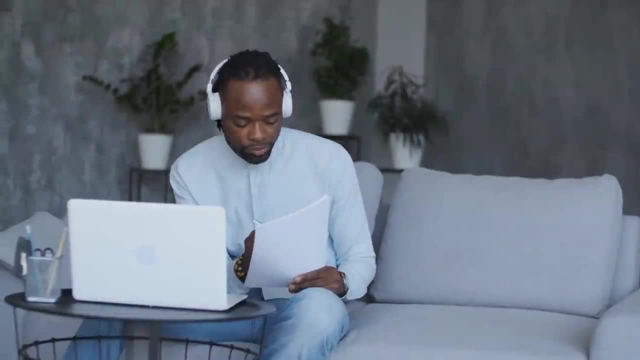 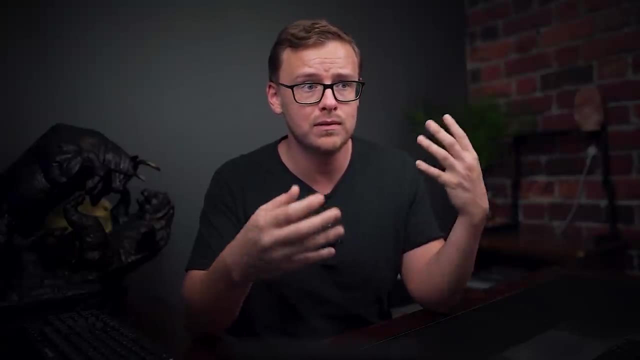 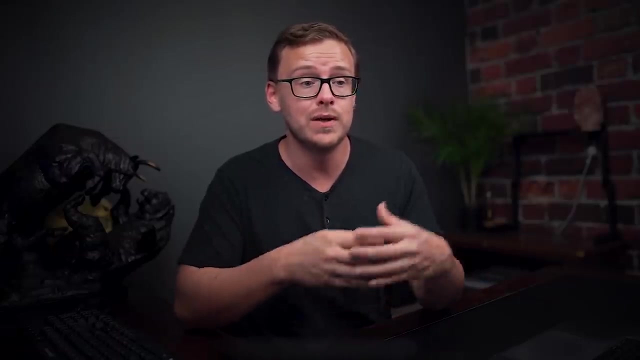 It's also surprisingly and ironically, cheaper in many cases to get one on one teaching from somebody than to actually go to college. where you're going to, you know have like 40 other students in a classroom to one teacher. No, seriously Like the amount of time that you spend in the classroom. 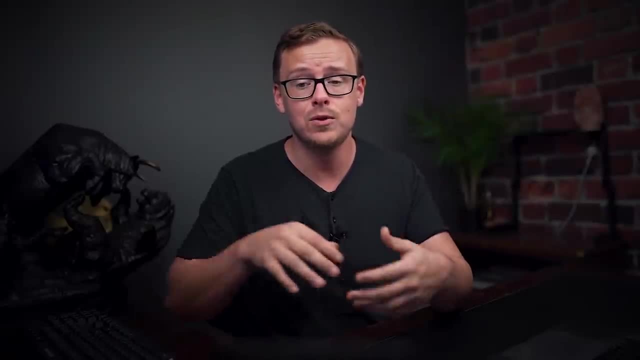 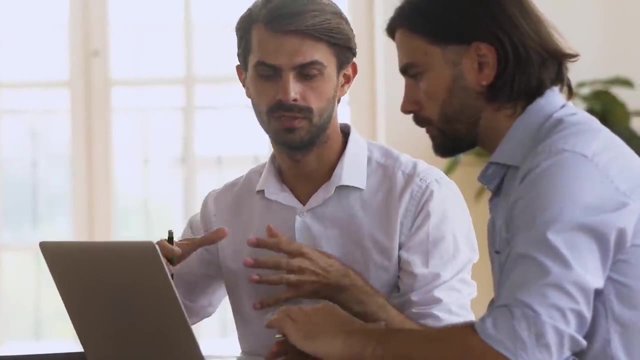 With a professor. If you just took that same amount of time, you could pretty easily in many cases just hire somebody who is a professional or who's really good at whatever skill you're trying to learn, to coach you one on one, And I'm not even kidding about that. 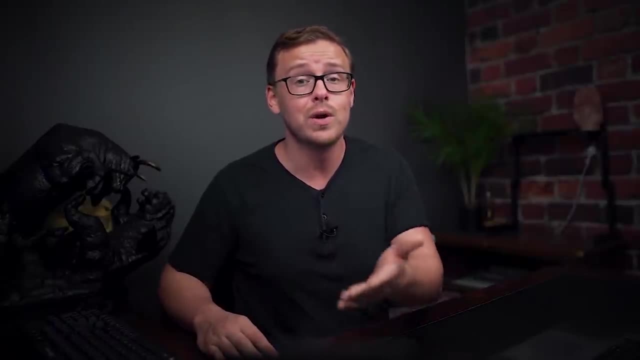 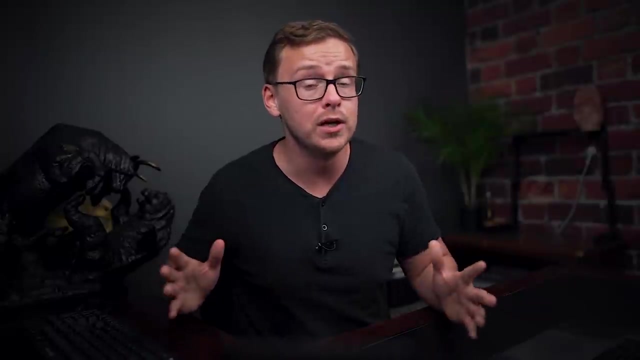 Like these. things are out there. They're available. You can look at websites like fiverrcom. There are people who posted on Facebook, Marketplace, Craigslist, etc. Right, So there's so many different ways for you to get educated. College is a great choice, depending on the career path you're going down. 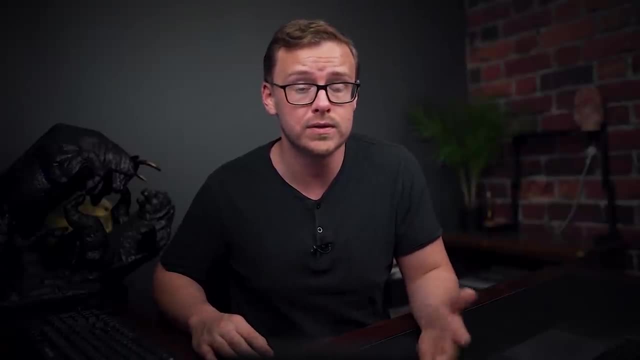 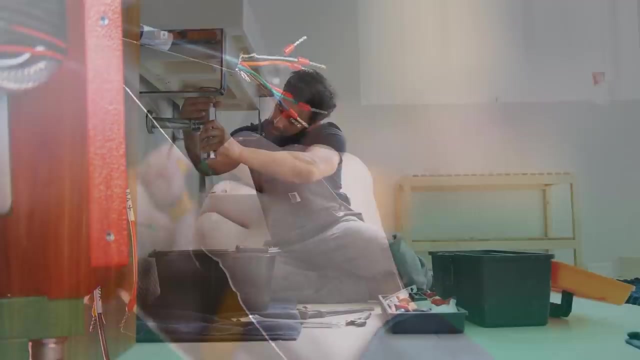 And then also just learning skills So you know another career path you could go down is trade Right, You could become a tradesman, an electrician, a plumber, HVAC mechanic, etc. These are skills that are very valuable.